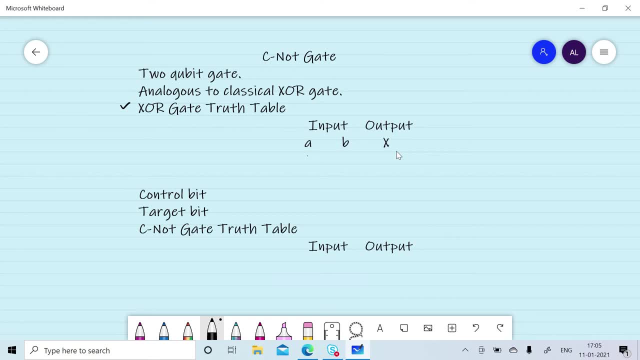 get 1 as the output. Otherwise we will get 0 as output. So, if input are 00, we will get 0 as the output. If input are 01, we will get 1 as the output. If we have input 10, we will get 1 as the. 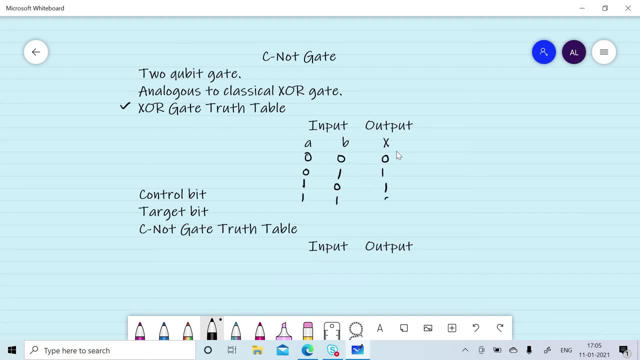 output. If we have 11 as the input, we will get zero as the output. So if exactly one of the input is one, we will get one as the output. We can also call A as a control bit and B as a target. 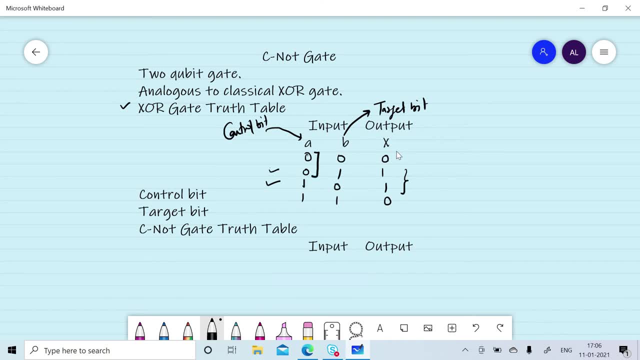 bit. If our control bit is zero, we will copy the value of b in the output. that is zero or one. If our control bit is one, we will flip the value of b as the output, Like if we have zero as the value. 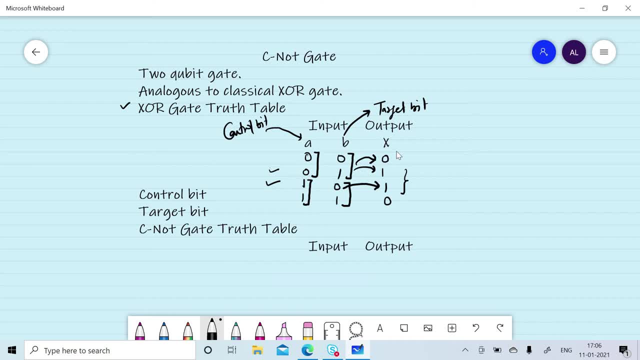 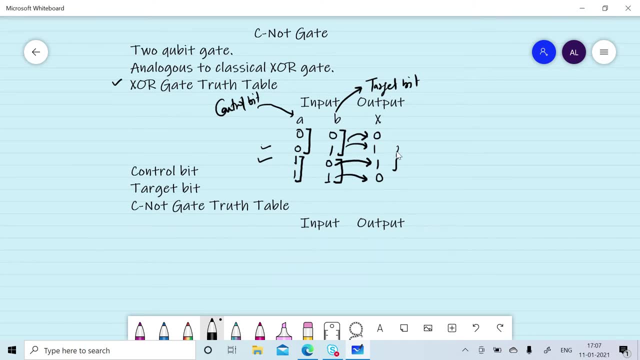 of b, we will flip it and we will get one as the output. If we have one as the value of b, we will flip it. we will get zero as the output. In the same way, in case of control, not gate, if we have. 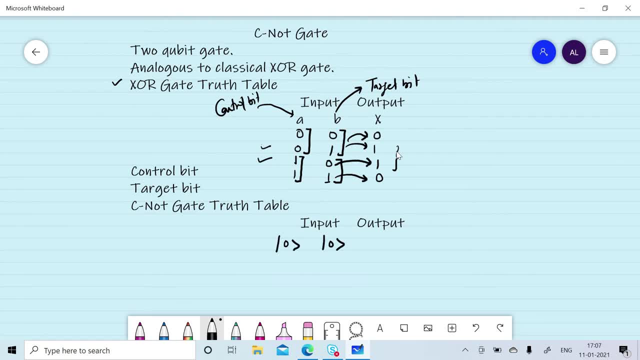 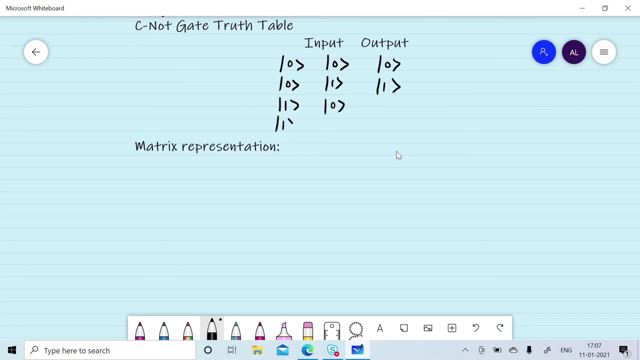 input qubit are in zero- zero state, we will get zero as the output. If we have zero one, we will get qubit in one state as the output. If input qubit are in one state and zero state. if input qubit in one state and the second qubit is also in one state, we will flip the value of second. 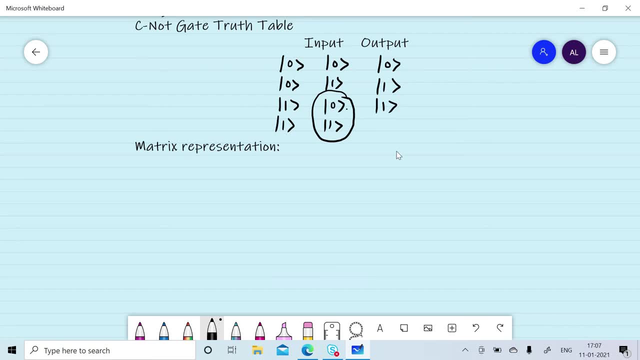 qubit, That is, we will get one. by flipping zero we will get one, and by flipping one we will get zero Again. the first qubit is known as control qubit and second qubit is known as target qubit. So if our control qubit is in zero state, we will copy the value of target qubit in. 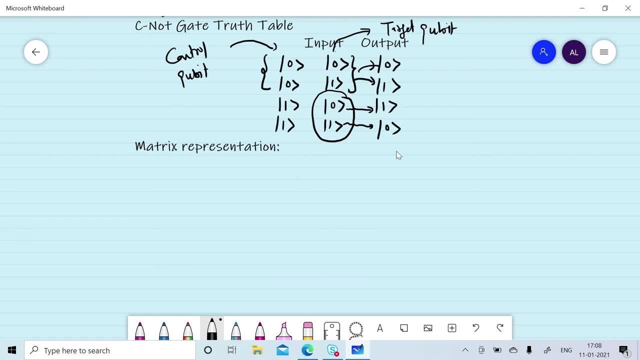 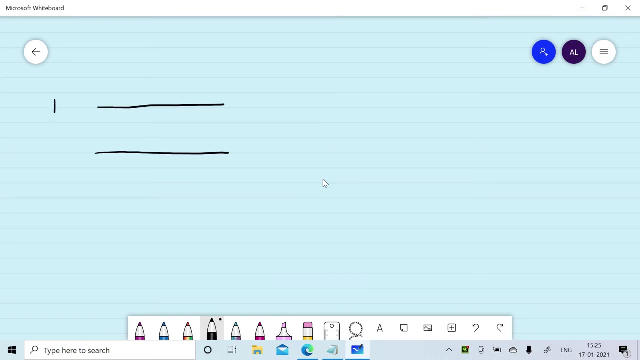 the output like zero one. If our control qubit is in one state, we will flip the value of target qubit as the output- C, not gate, can be represented by. consider: the control bit is represented by A and target bit is represented by B, So C, not, is represented. 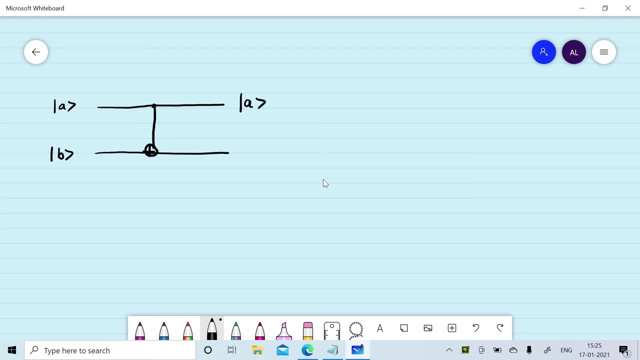 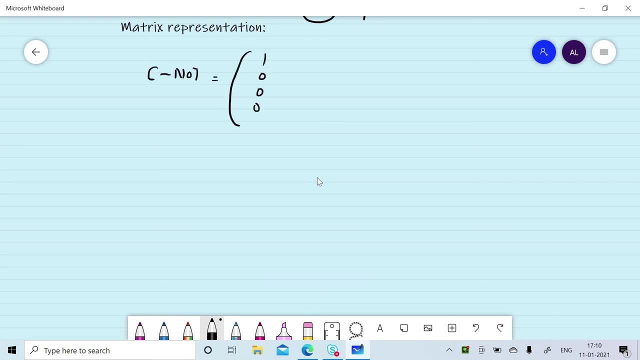 by and we will get output as A and A bit, B, C, not gate, can be represented by one zero zero, zero, zero, one zero, zero, zero, zero, zero, one, zero, zero, one zero. And if our input are zero, zero, that is, first qubit is in zero state, second qubit is in zero state- we can represent it by one zero zero. 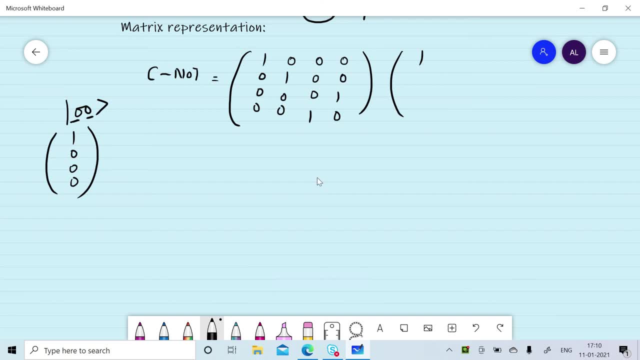 zero. So if our qubit in zero zero state, so it is one zero, zero, zero, we will get output as one zero, zero, zero. Similarly, if our input is in zero one state, so we have zero, one, zero, zero, because the second row will represent zero one entry. 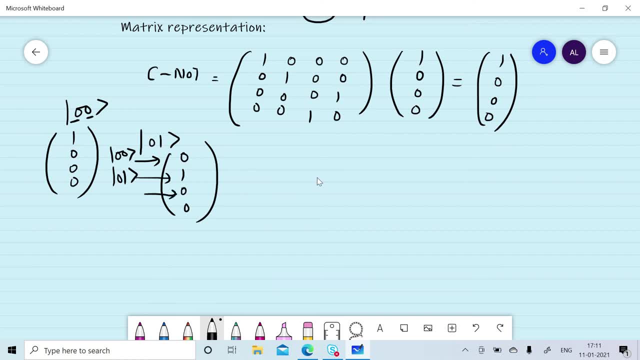 So the first row will represent zero, zero state and the third row will represent one zero state and fourth row will represent one one state. So if our input are zero, one, zero, zero, that is zero one state. so we will get output as zero one. So it is again zero one state. First zero will. 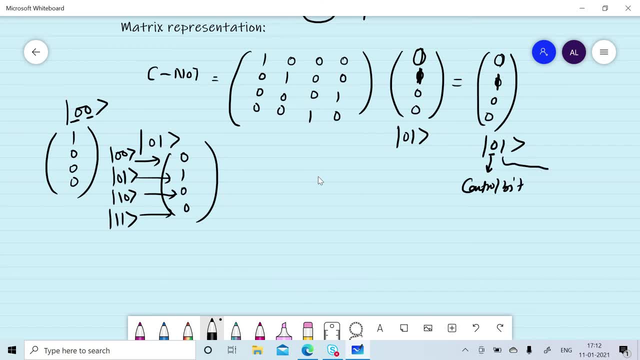 represent the control bit and second bit represents the outcome of the C, not gate. Similarly, if our input are zero, one zero, zero, zero, zero. that is, we have one zero state that is first qubit in one state and second qubit in zero state. we can represent it by zero, zero, one zero And after. 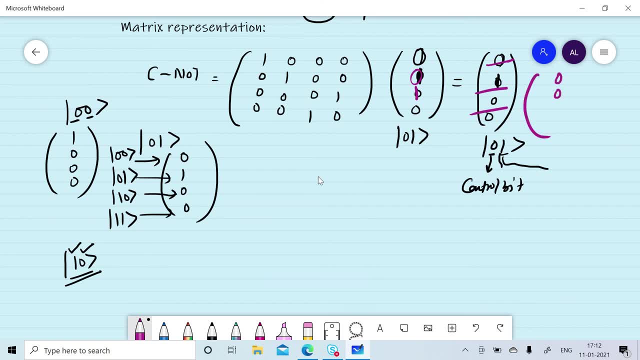 applying C not gate, we will get zero, zero, zero one. that is one, one state. So in case of C not gate, if we will give zero, zero as the input state of two qubit, we will get zero, zero as the output. 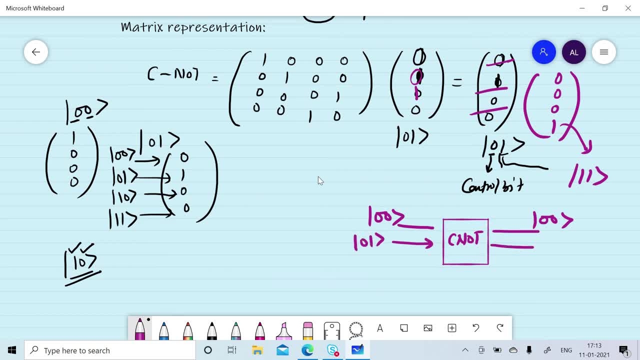 If we will give input as 01,, we will get 01 as the output state of 2 qubit. If we will give 10 as the input, we will get 11 as the output state of the 2 qubit. Similarly, if we will give 2 qubit in 11 state, we will get the output state as 10,. that is flipping of target bit.